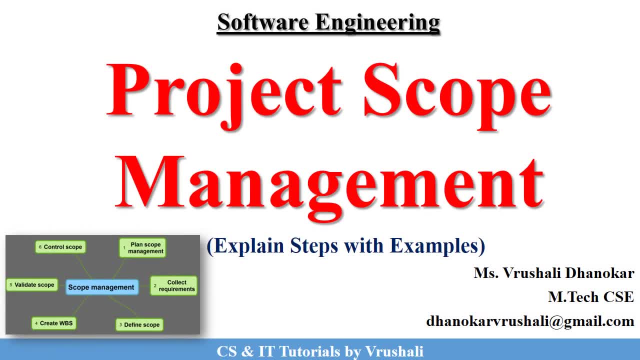 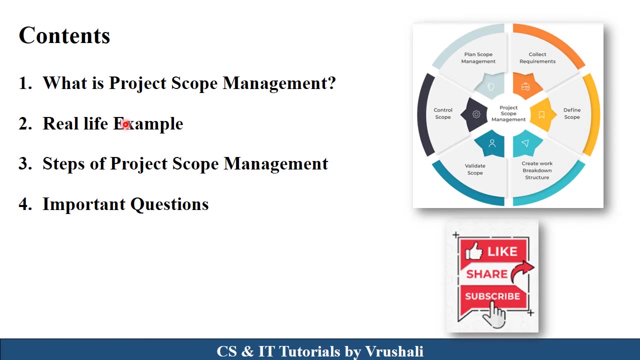 Hello everyone. this is Vrishali. In previous session we discussed project planning process with examples. I have mentioned complete software engineering subject playlist link in below description box. Now in today's session we will discuss the next important topic, that is, project scope management. Let's start the session. In this session we will discuss what 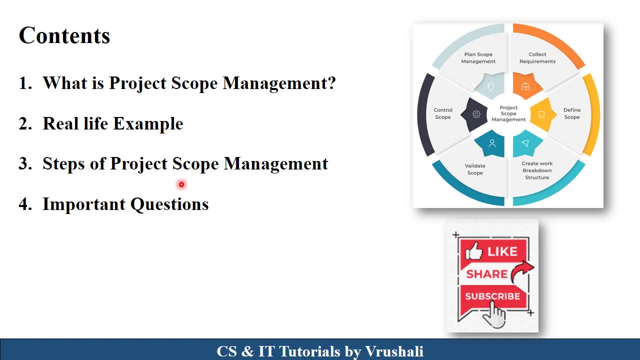 is project scope management, real life example, steps of project scope management and some important questions that have asked in previous year question paper. Let's see all these points one by one Now. the first thing is: what exactly project scope management? First, we understand. 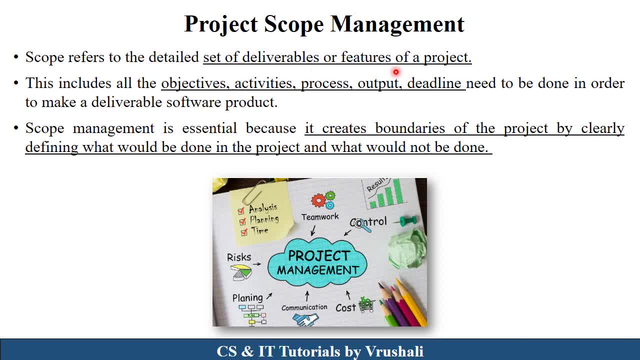 what is scope? Scope means set of deliverables or features of particular project. For example, the particular project include objective, different activities, different process, output and deadline- This kind of features. So this set of features are called as scope. Now, what is scope management? 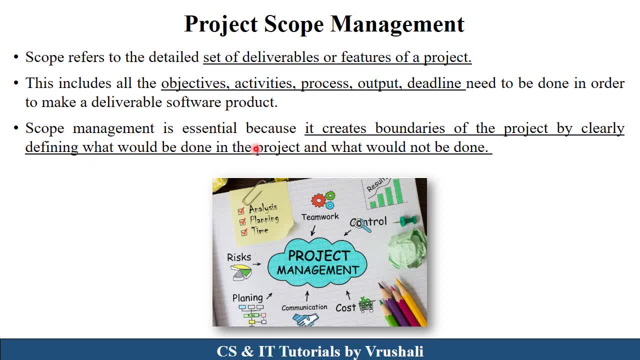 So basically, scope management decide what would be done in particular project and what would not be done. Basically it create a boundaries means which information required in particular project and which information is not required in particular project. So this thing has decided in the planning phase. This is called as scope management. Let's see here in this example: 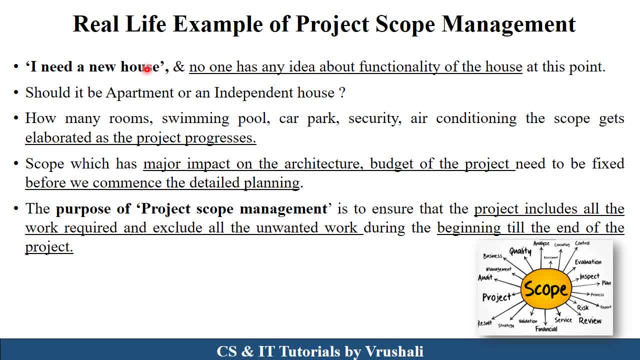 suppose someone said I need a new house, But this sentence does not generate. should it be apartment or independent house, Right Or no one has any idea about functionality of the house. So the functionality include how many rooms, swimming pool, car parking. 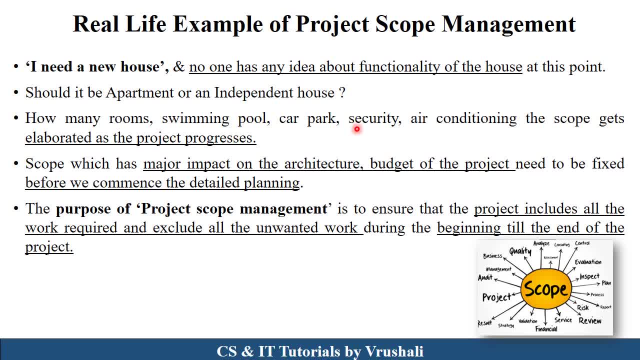 security, air conditioning Right. So this set of features are called as scope. Scope also elaborate progress of particular project, And scope also impact on architecture, design, architecture budget and timeline of particular project. So basically, the main purpose of project scope management is to decide which information is required and which information. 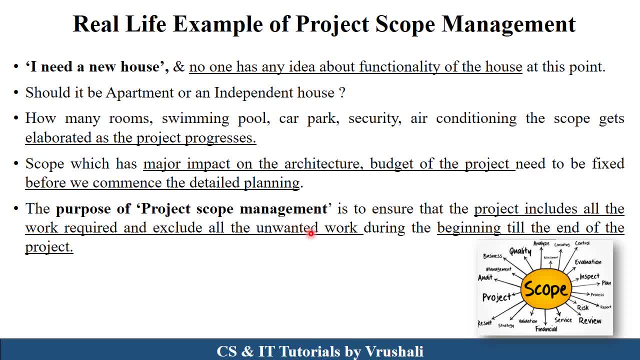 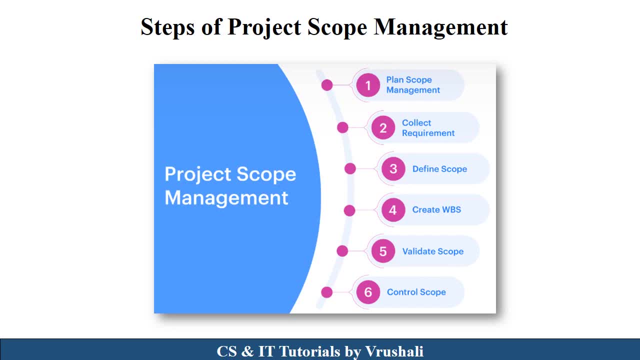 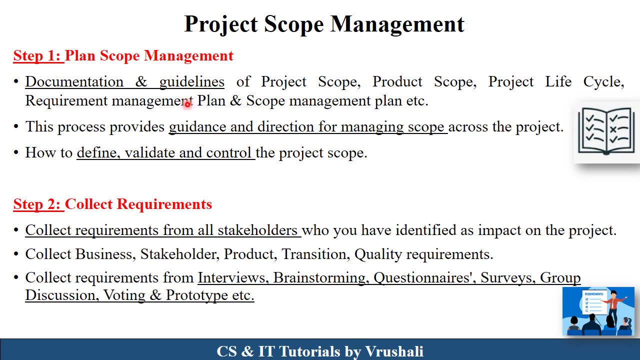 not required in particular project. So here, project manager decide all those things at the beginning of particular project. So this is the importance of project scope management. In project scope management there are total six steps. Let's discuss all the steps in detail. The first step in project scope management is plan scope management. In this first step, 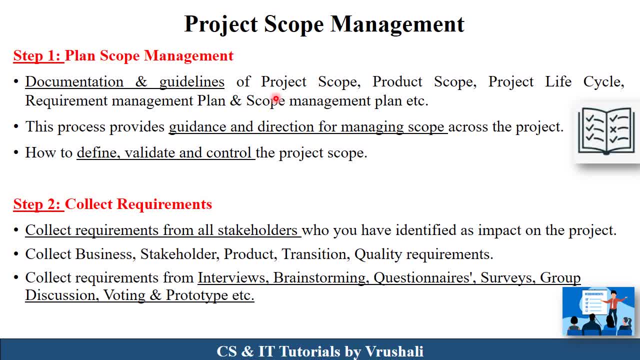 there is just guidelines or documentation related to how to generate project scope, product scope, how to create project life cycle- means software development life cycle- which type of models are used then, how to decide requirement management plan, scope management plan. So all the guidelines related to all those things are mentioned in one document. 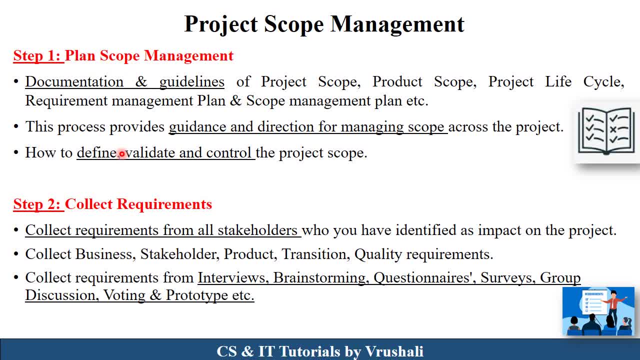 So these documents are called as plan scope management. They define, validate and control a complete project scope. Now in second step is to collect requirements. Here the first importance is for the customer, So collect requirement from the all the stakeholders. There are different types of requirements, like business stakeholder, product transaction. 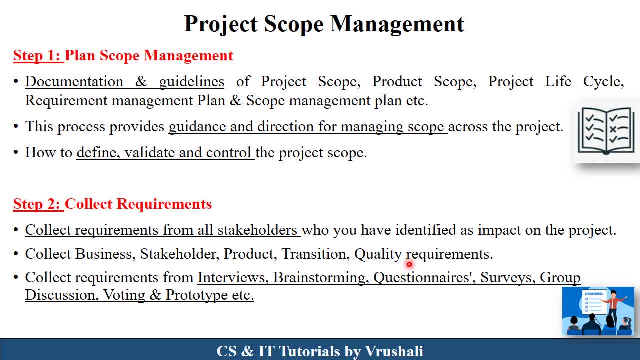 and quality requirements. You can use different requirement collecting methods, like you need to collect interview, brainstorming session, questionnaire and other requirements. So you can use different requirement collecting methods, like you need to collect interview, brainstorming session, questionnaire, survey, group discussion, voting and prototype. So 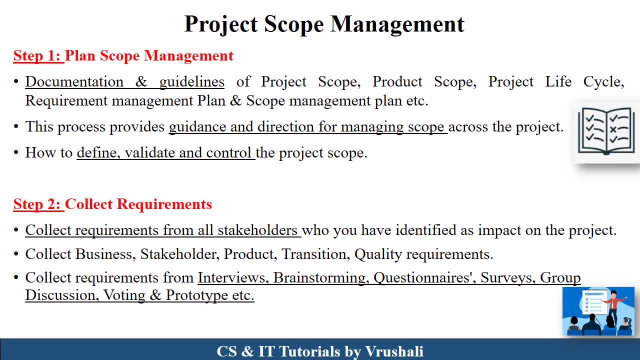 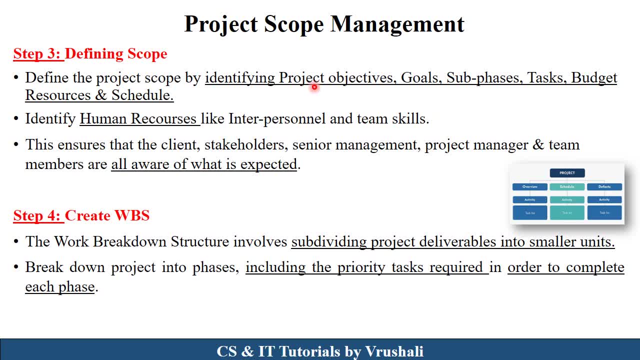 you can use these all methods for collecting requirements from the customer. The third step is defining scope. Here you need to define what is the objective, what is the goal of particular project, why particular project, particular product have developed Different sub phases, task budget, which type of resources, like software resources. 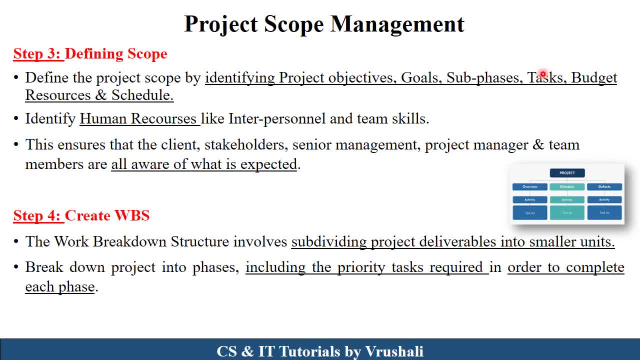 hardware resources and schedule of particular project. These all things have defining in particular scope. They also identify human resources means which team is required for developing a particular project, which type of skills, which type of specialty have required. So all the stakeholders are aware, by using all 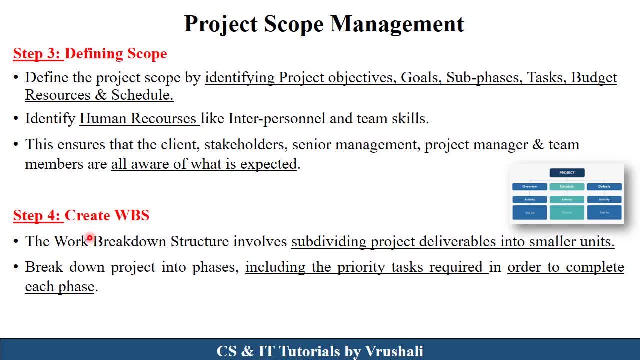 this scope of particular project. The next step is create WBS. WBS means work breakdown structure, Basically before designing and developing phase. In planning phase, the complete project have divided into the smaller units, or we can say different modules, and they also decide which type of modules having highest priority means. 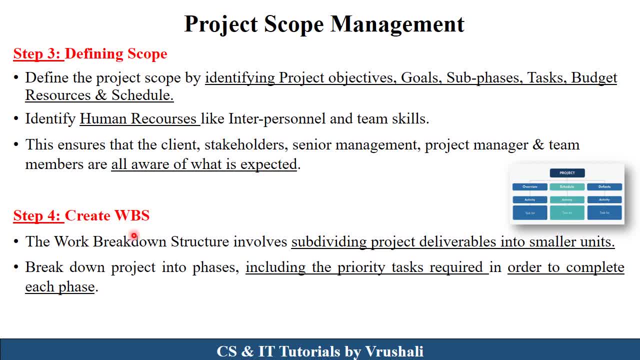 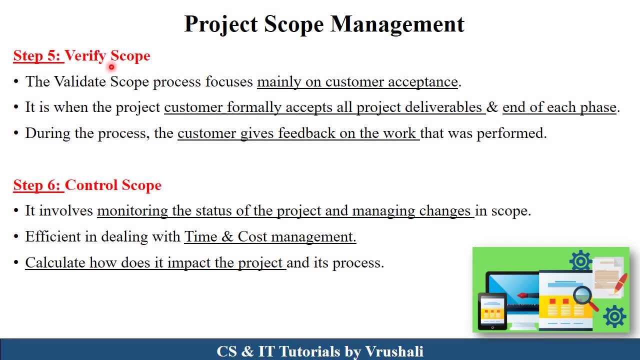 which module customer required first. So this is called as work breakdown structure. In our next session we discuss work breakdown structure in detail with example. So basically it divide a complete project into the smaller units. The next step is verify scope. So verify scope means that you need to know the scope of the